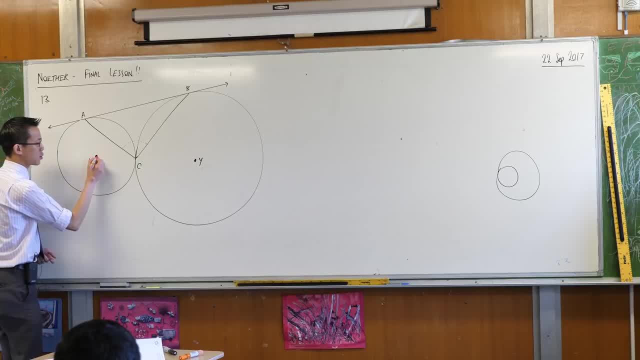 I'm going to put these radii in as the same colour, because then it's sort of like a whoops, sorry, it should go. oh, that's terrible. It's sort of a visual cue for me that these things are the same and I can see it instantly right. 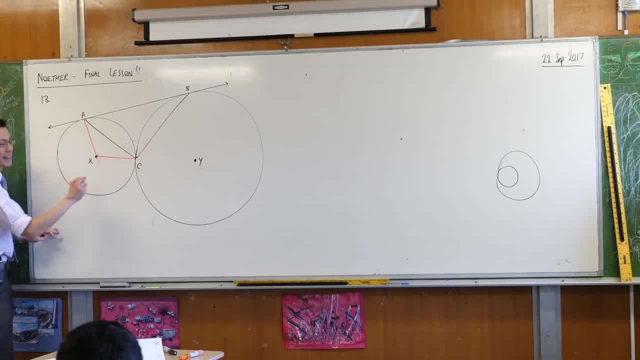 I know you can, I know you can add like a little dash to say, oh, these things are the same, but often those dashes kind of get lost in the mix. okay, So there's a pair of equal radii. 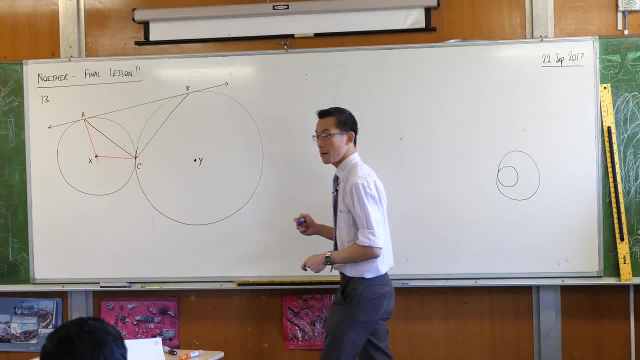 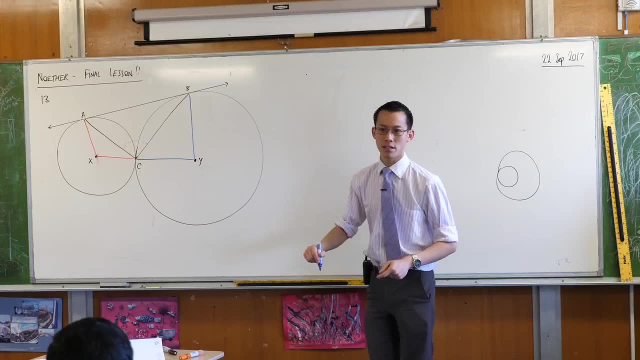 What were the other ones you were going to put on, C Y and B Y, fantastic. So, just like before, I'm going to put these guys in the same colour, but you notice it's a different colour to the other ones, because these are well, they're different size circles, okay. 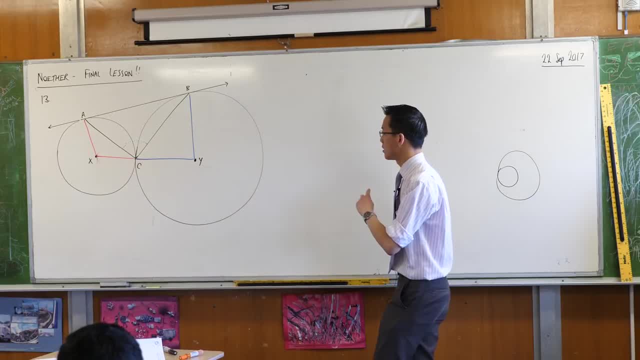 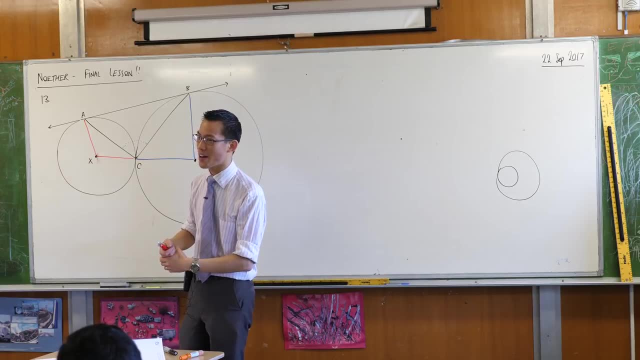 Right now, staying with these colour themes. when you've created these radii, you have created triangles. Do you notice that? This is familiar, right? What kinds of triangles have you created? Isosceles triangles, right? So I'm going to get equal angles going around. 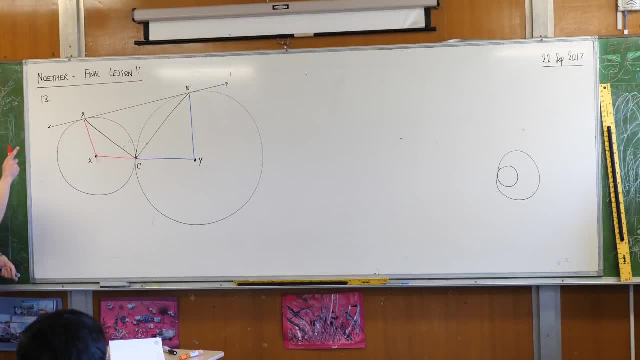 I might start naming some. so, for example, in triangle AXC, which are the equal angles, Which, what are the names? XAC is one of the base angles and XCA that one there. okay, So let's just give them a name. I'm just thinking here. right, If this is alpha, then we'll make this one alpha as well, okay? 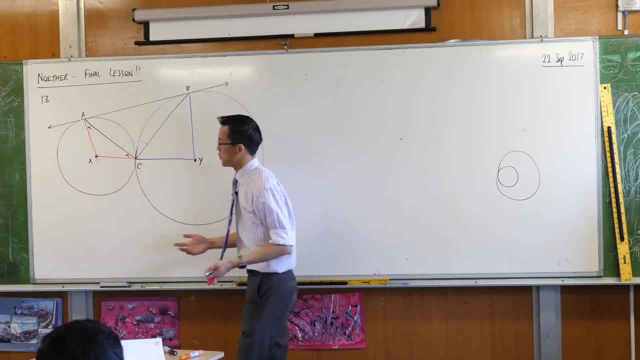 On the right-hand side of the bigger circle. I mean, I've used alphas. what would you like me to call the angles in this triangle? How about beta? So you've got base angles here and here. okay, Now what else do you know about this? 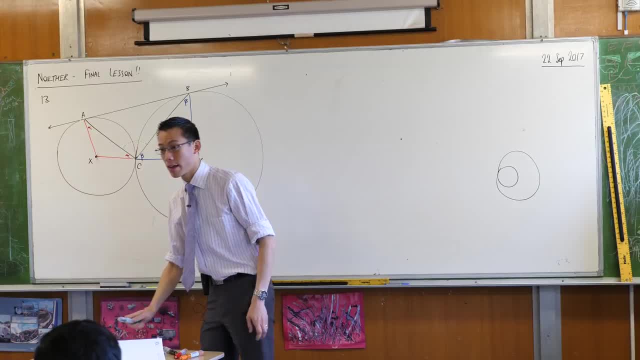 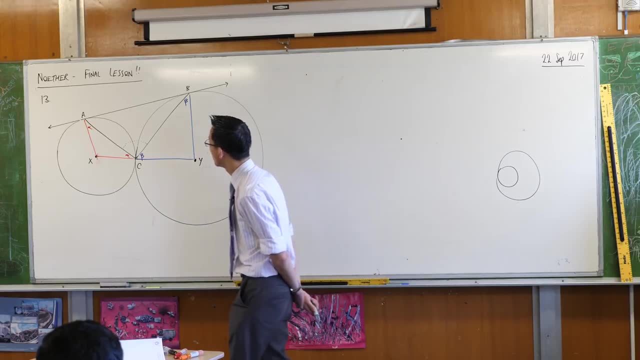 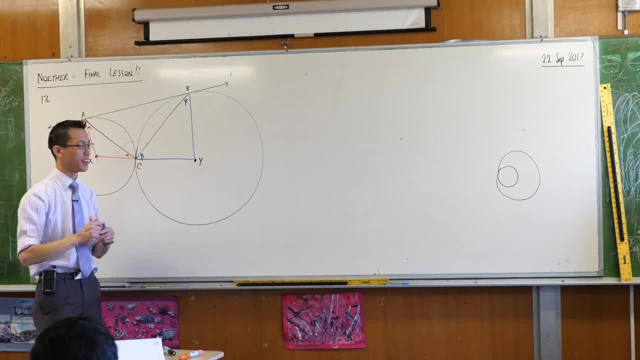 C, A and B is 90 minus 90.. Okay, so we're going to suggest that this guy up here. I'll go back to my alpha color. We're suggesting that this is 90 degrees minus alpha. but we actually need to take a step back first to realize why that's the case. 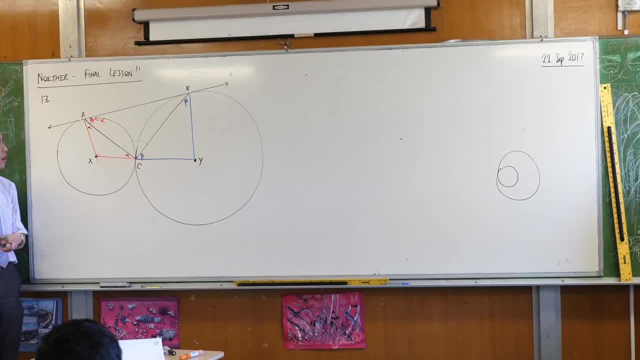 Why is that? 90 minus alpha? Because AB is a tangent. Okay, if AB is a tangent, then it's perpendicular to the radius of the point of contact. Does that make sense? So actually there is a right angle here, And so that's why you've got right angle: alpha 90 minus alpha 90.. 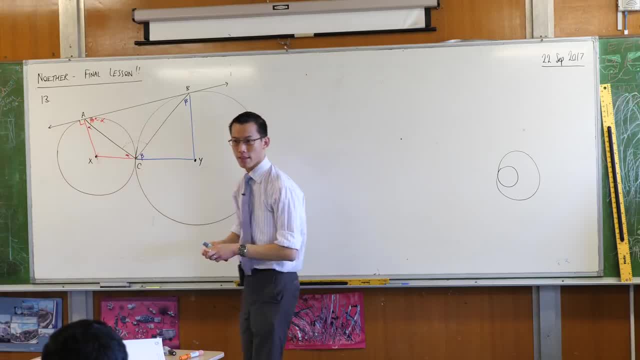 Alpha, they all add up to 180.. Same thing happening over here, right? Where's the 90 minus beta? A B C. A B C is 90 minus beta, for the same reason, So let me just mark that in. 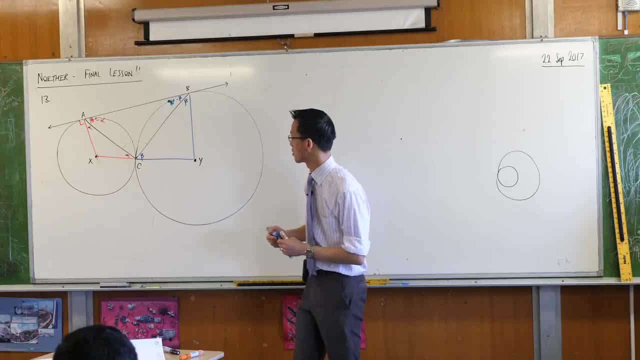 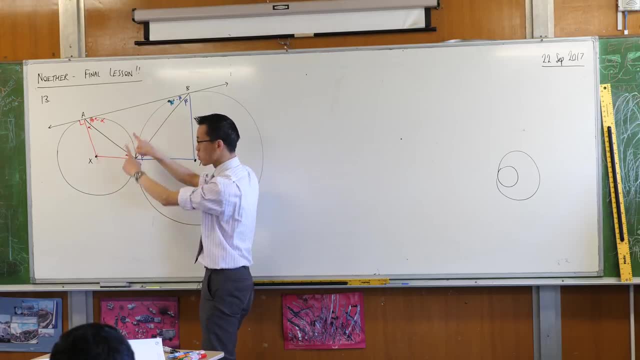 Now, at this point we're super, super close. We're very, very close. If I've got two angles in this ABC triangle- the biggest one that I've got here- then the two angles will give me the third angle, right. 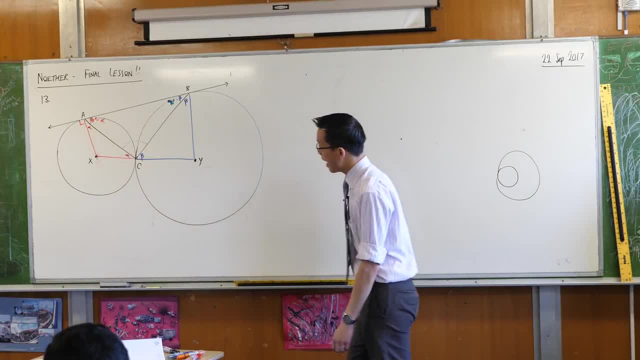 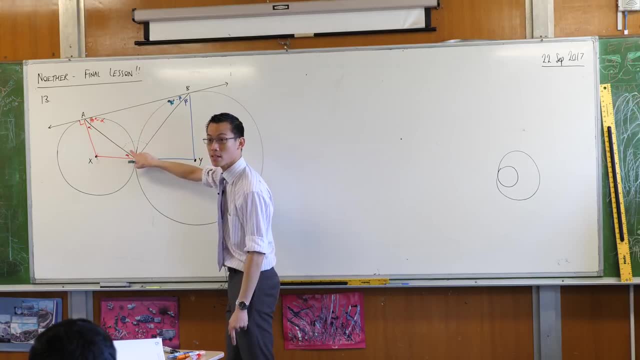 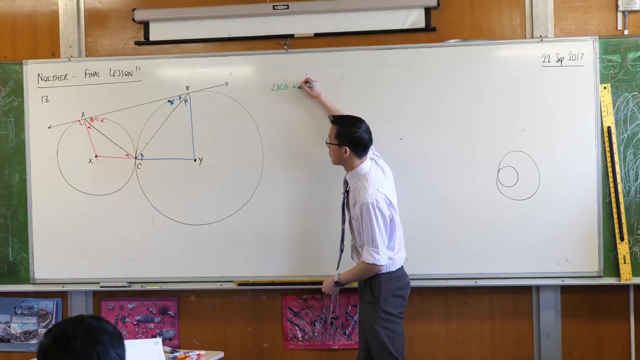 What is this third angle? If the angle of a triangle is 180 degrees, then this plus this, plus this mystery angle- let's actually write this out- ACB is our mystery angle plus BAC, which you know is 90 minus alpha. 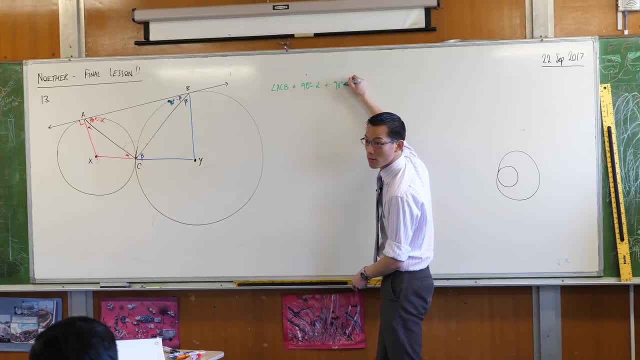 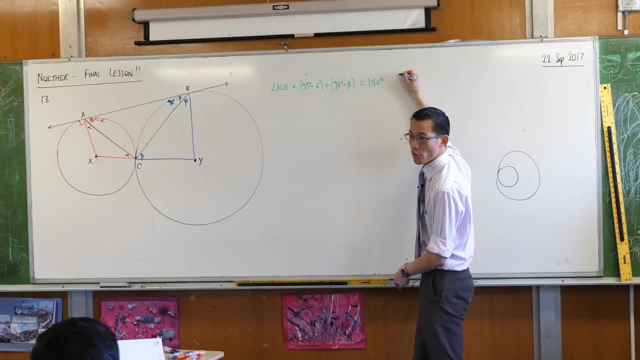 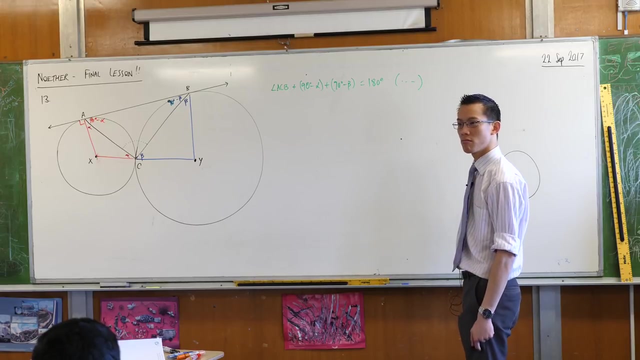 and ABC, which is 90 minus beta. right, These guys are all equal to 180 degrees And you have your reason for this, right? Angle sum of triangle, ABC- yep, Okay. so what can I do with this? 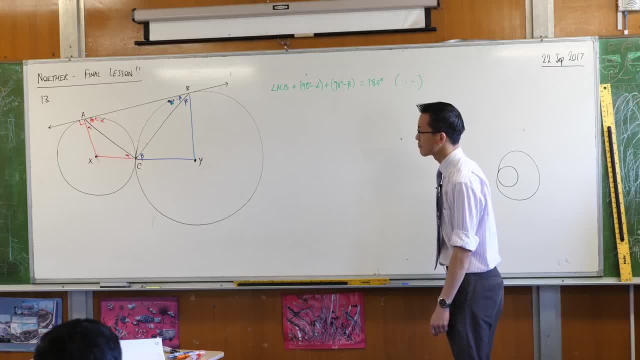 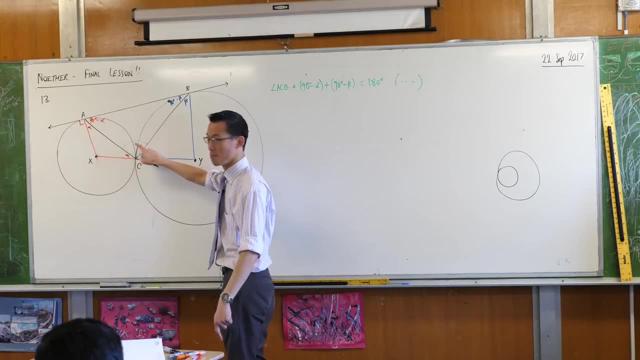 Can you write ACB as 180 minus alpha plus beta, This one here, Yeah, Yeah, I could do that. I'm going to come to that in a second, but this is what we sort of pointed out before, so I'll come back to your line of logic in a minute. 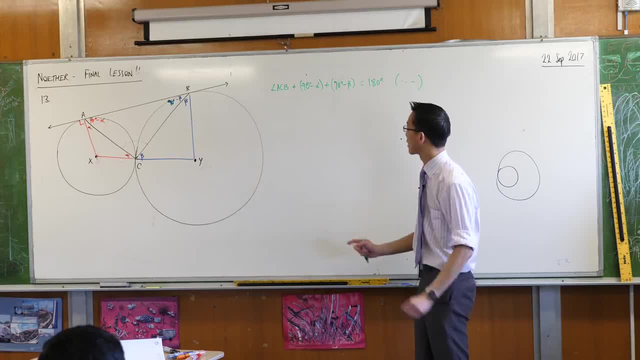 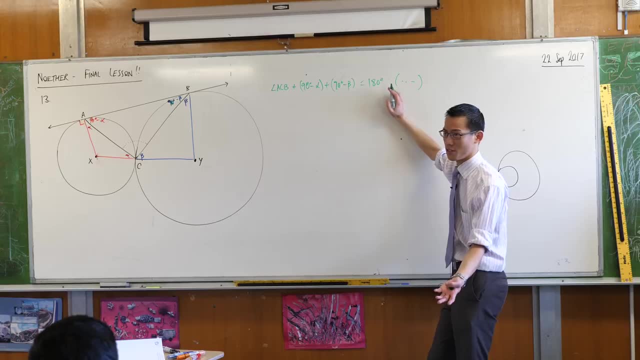 because it's just two ways around the same obstacle. okay, Have a look. Look at the angles right, So can you see you've got 90 and 90 here and a 180? So what could I do to both sides that might make this nice and simple? 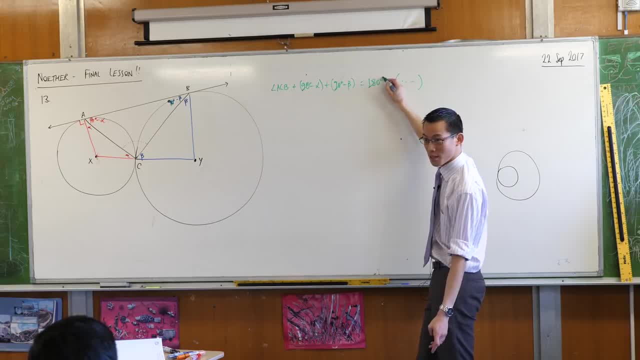 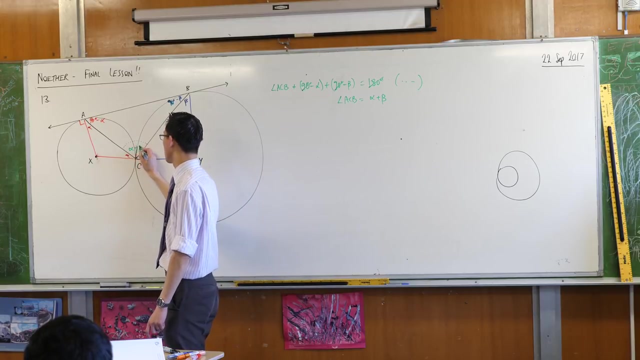 I could just Yeah. once I subtract these and add alpha plus beta to both sides, you get ACB being alpha plus beta, Is that okay? So this mystery angle, I can say either the way that Roger stated it or the way that we've stated it just now, that's alpha plus beta, okay.